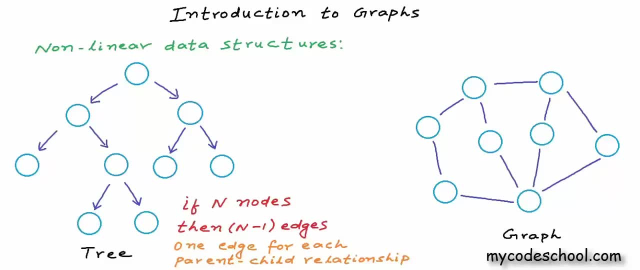 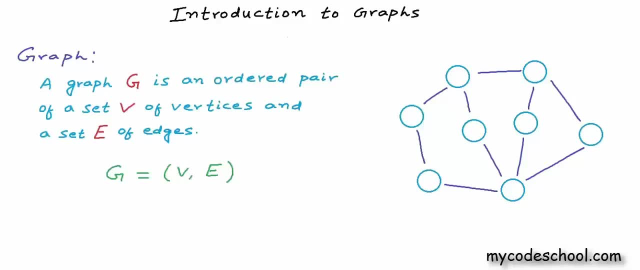 among the nodes. So in a tree there are rules dictating the connection among the nodes. Now we can define graph something like this: a graph G is an ordered pair of a set v of vertices and a set e of edges. Now I am using some mathematical jargon here. An ordered 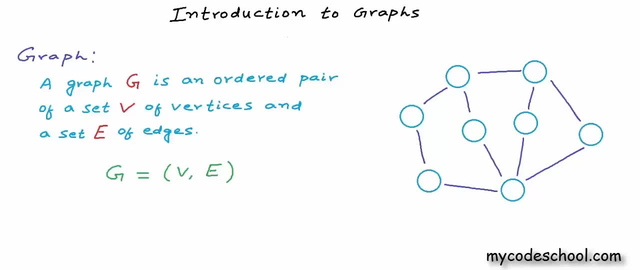 pair is just a pair of mathematical objects in which the order of objects in the pair matters. This is how we write and represent an ordered pair: Objects separated by comma, put within parentheses. Now because the order here matters. Now because the order here matters. 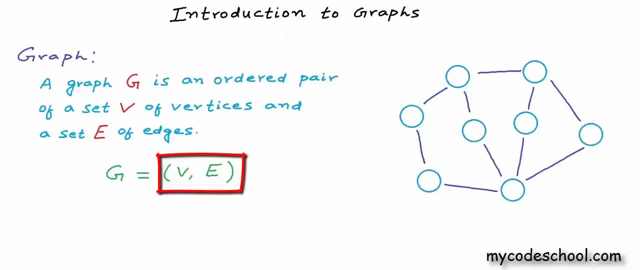 Now, because the order here matters pairs, we can say that V is the first object in the pair and E is the second object. An ordered pair. AB is not equal to BA unless A and B are equal In our definition of graph. here first object in the pair must always be a set of vertices and the second object 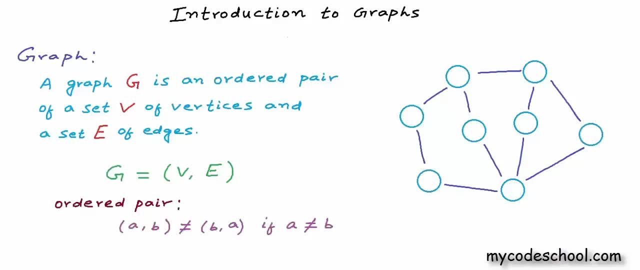 must be a set of edges. That's why we are calling the pair an ordered pair. We also have concept of unordered pair. An unordered pair is simply a set of two elements. Order is not important here. We write an unordered pair using curly brackets or braces, Because 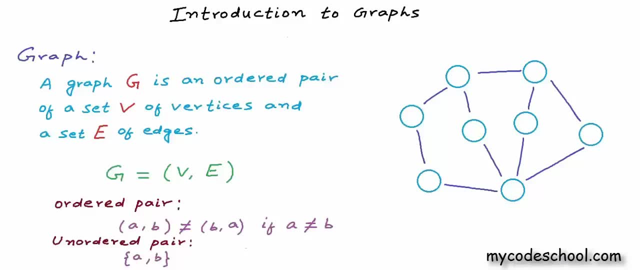 the order is not important here. unordered pair AB is equal to BA. It doesn't matter which object is first and which object is second. Okay, coming back, so a graph is an ordered pair of a set of vertices and a set of edges and G equal VE is equal to BA. So 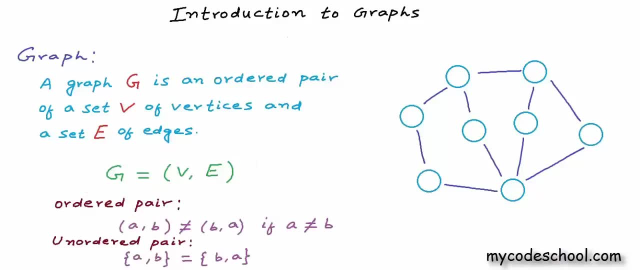 VE is a formal mathematical notation that we use to define a graph. Now I have a graph drawn here in the right. This graph has 8 vertices and 10 edges. What I want to do is I want to give some names to these vertices, Because each node in a graph must have some. 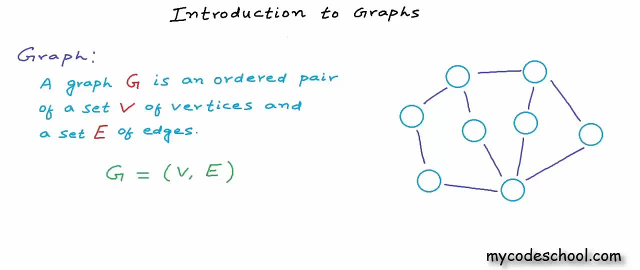 identification. It can be a name or it can be an index. I am naming these vertices as V1, V2, V3,, V4, V5 and so on, And this naming is not indicated. There is no first, second and third node here. I could give any name to any node, So my 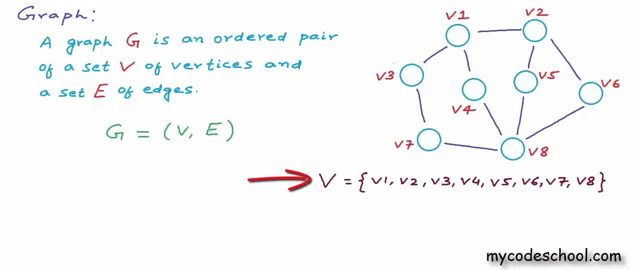 set of vertices here is this. We have 8 elements in the set: V1,, V2,, V3,, V4,, V5,, V6,, V7 and V8.. So this is my set of vertices for this graph. Now what's my set of edges? To answer, 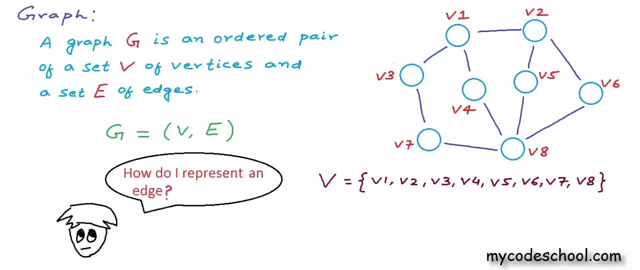 this, we first need to know how to represent an edge. So we can just write the names of the two end points of an edge as a pair and it can be a representation for the edge. But edges can be of two types. We can have a directed, 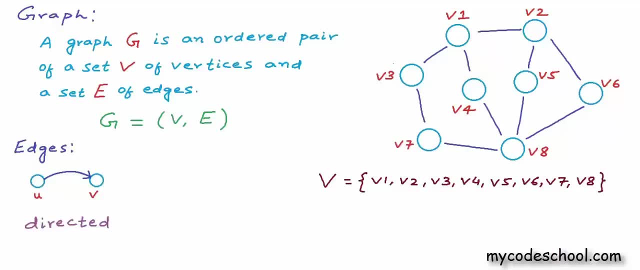 edge, in which connection is one way. or we can have an undirected edge, in which connection is two way. In this example graph that I am showing here, edges are undirected, But if I assume the basic Machine Learning in the tree and this side that I had shown earlier, 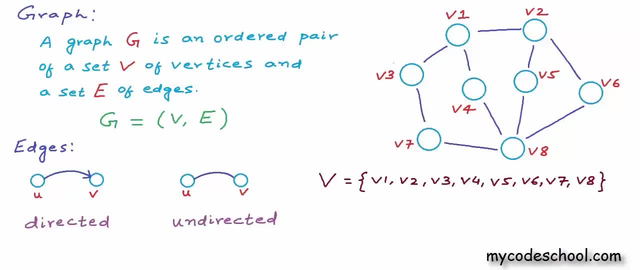 then we have directed edges in that tree. With this directed edge that I am showing you here, we are saying that there is a link or path from vertex U to V, But we cannot assume a path from V to U. This connection is one way For a directed edge. 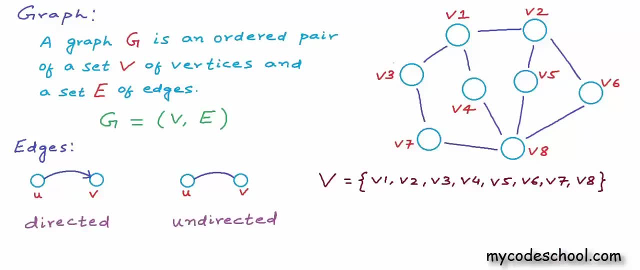 one of the end points would be the origin and the other end point would be destination. For our edge here, origin is U and destination is V. A directed edge can be represented as an ordered pair. First element in the pair can be the origin and second element 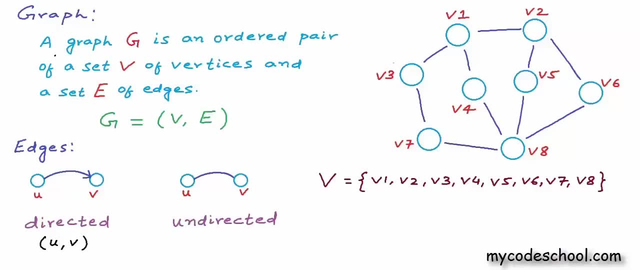 can be the destination. So with this directed edge represented as ordered pair, UV, we have a path from U to V. If we want a path from V to U, we need to draw another directed edge here, with V as origin and U as destination, And this edge can be represented as ordered. 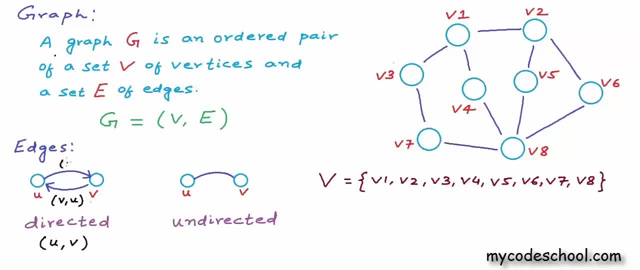 pair VU. The upper one here is UV and the below one is VU, And they are not same. Now, if the edge is undirected, the connection is two way. An undirected edge can be represented as an unordered pair Here, because the edge is bidirectional. origin and destination are 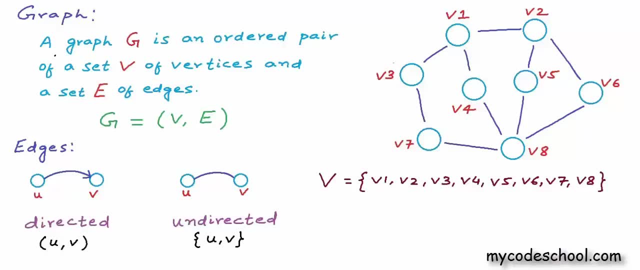 not fixed. We only need to know what to do. So now that we know how to represent edges, we can write the set of edges for this example graph. here We have an undirected edge between V1 and V2.. Then we have one between V1 and. 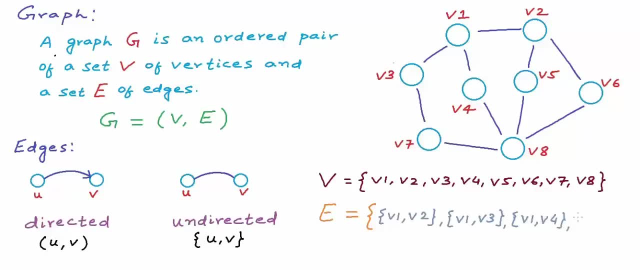 V3.. Then we have V1,, V4. This is really simple. I will just go ahead and write all of them. So this is my set of edges. Typically in a graph, all edges would either be directed or undirected. It's possible for. 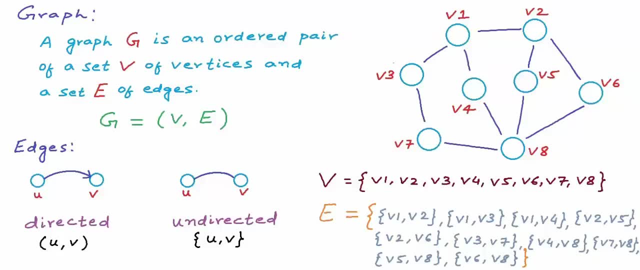 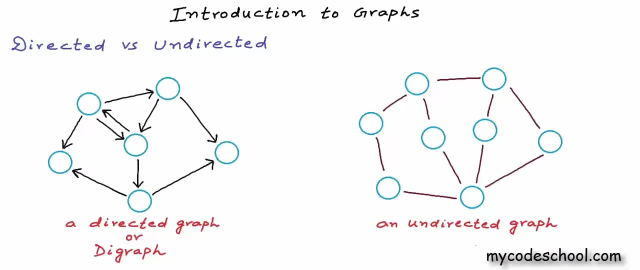 a graph to have both directed and undirected edges, But we are not going to study such graphs. We are only going to study graphs in which all edges would either be directed or undirected. A graph with all directed edges is called a directed graph or digraph, And 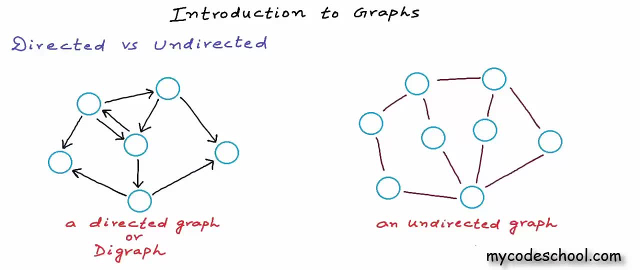 a graph with all undirected edges is called an undirected graph. There is no special name for an undirected graph. Usually, if the graph is directed, we explicitly say that it is a directed graph or digraph. So these are two types of graph: Directed graph or digraph. 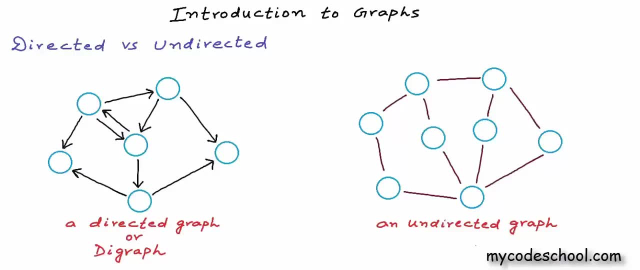 in which edges are unidirectional or ordered pairs, and undirected graph in which edges are bidirectional or unordered pairs. Now, many real world systems and problems can be modelled using a graph. Graphs can be used to represent any collection of objects having 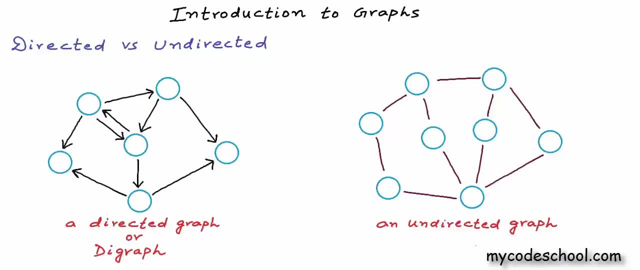 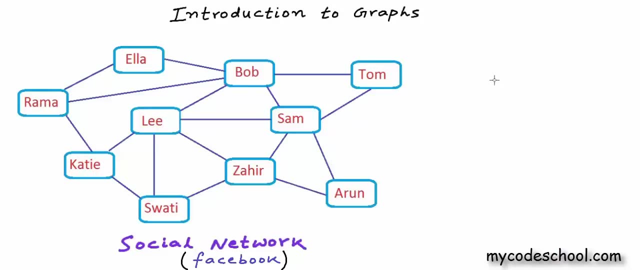 some kind of pairwise relationship. So what is a pairwise relationship? A pairwise relationship is a relationship between two users. Let's have a look at some of the interesting examples. A social network like Facebook can be represented as an undirected graph. A user would be a node in the graph, and if two users 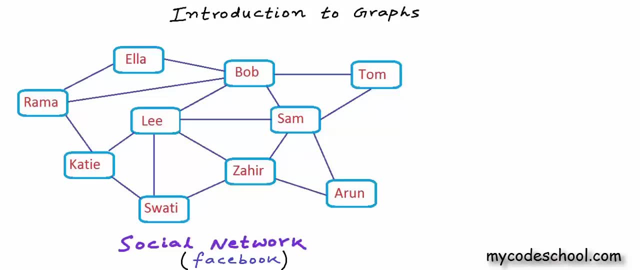 are friends, there would be an edge connecting them. A real social network would have millions and billions of nodes. I can show only few in my diagram here because I am short of space Now. social network is an undirected graph because friendship is a mutual relationship. If I am your, 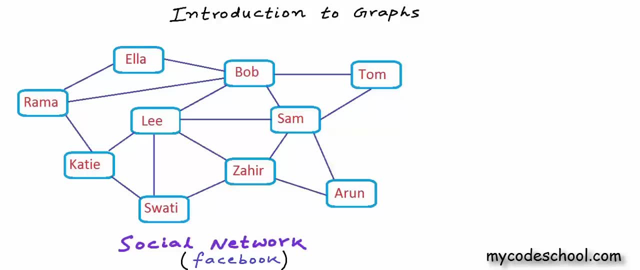 friend, you are my friend too, So connections have to be two-way. Now, once a system is modelled as a graph, a lot of problems can easily be solved by applying standard algorithms in graph theory, Like here in this social network. let's say we want to do something like suggest: 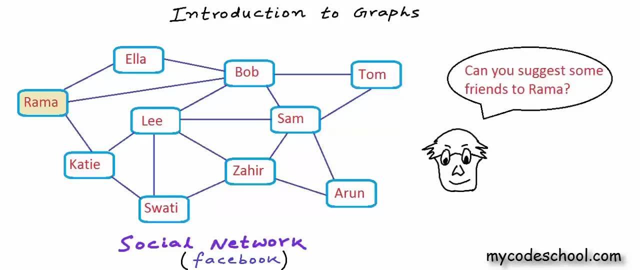 friends to a user. Let's say we want to suggest some connections to Rama. One possible approach to do so can be suggesting friends of friends who are not connected already. Rama can be suggested. Rama has three friends, Ella, Bob and Katie, and friends of these three that. 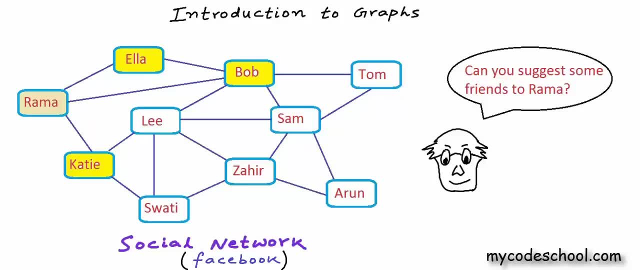 are not connected to Rama already can be suggested. There is no friend of Ella which is not connected to Rama already. Bob, however, has three friends, Tom, Sam and Lee- that are not friends with Rama, So they can be suggested, and Katie has two friends, Lee and Swati, that are not connected. 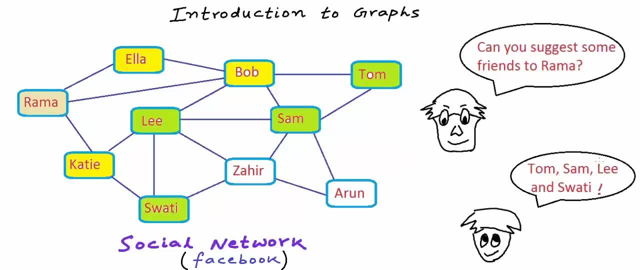 to Rama. We have counted Lee already, So in all, we can suggest these four users to Rama. Now, even though we described this problem in context of a social network, this is a standard graph problem. The problem here, in pure graph terms, is finding all nodes. 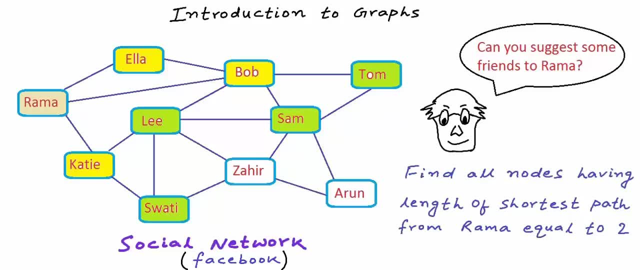 having length of shortest path from a given node equal to 2.. Standard algorithms can be applied to solve this problem. We will talk about concepts like path in a graph in some time. For now, just know that the problem that we just described in context of a social network. 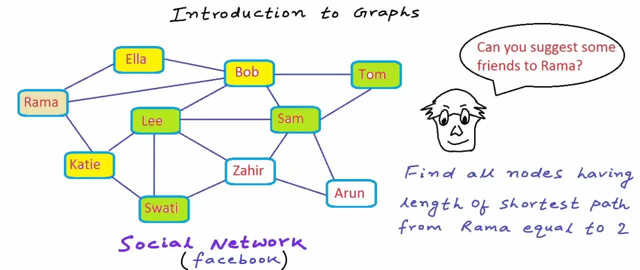 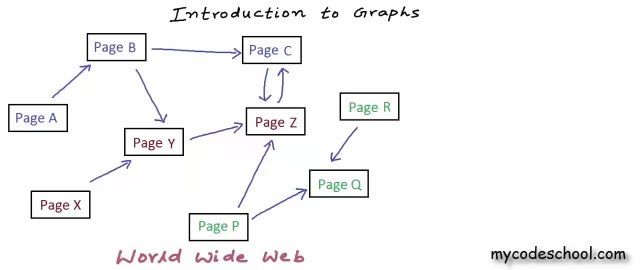 is a standard graph problem. Okay, so a social network like Facebook is an undirected graph. Now let's have a look at another example. Interlinked web pages on the internet or the world wide web can be represented as a directed graph. A web page that would have a unique 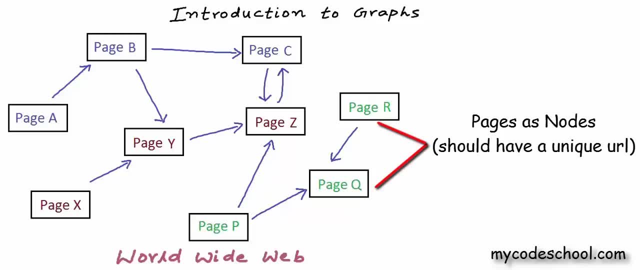 address or URL would be a node in the graph and we can have a directed edge if a page contains link to another page. Now, once again, there are billions of different ways to find pages on the web, but I can show only few here. The edges in this graph are directed. 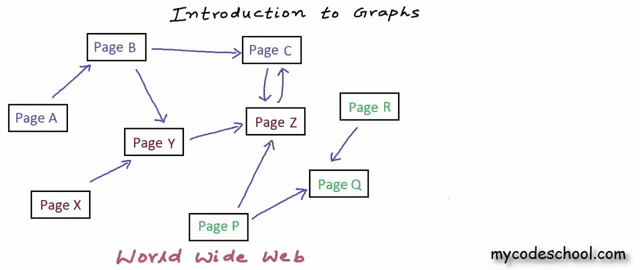 because the relationship is not mutual this time. If page A has a link to page B, then it's not necessary that page B will also have a link to page A. Let's say, one of the pages on mycodeschoolcom has a tutorial on graph and on this page I have put a link to Wikipedia. 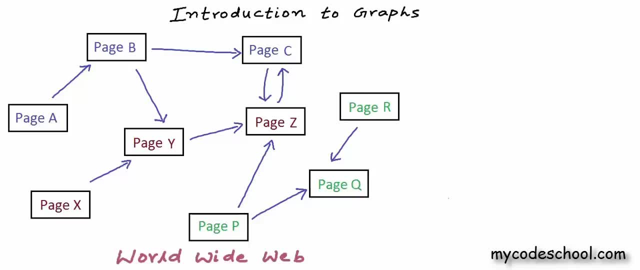 article on graph. Let's assume that in this example graph that I am showing you here, page B is my mycodeschool tutorial on graph, with this address or URL: mycodeschoolcom slash videos, slash graph. and let's say, page Q is the Wikipedia article on graph with this URL: 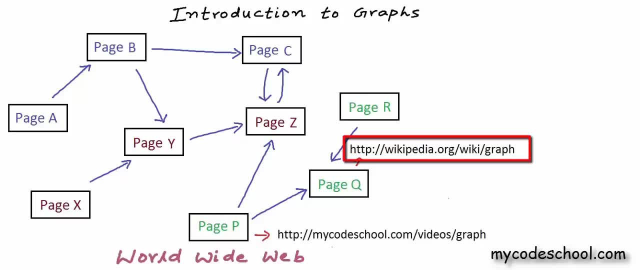 wikipediaorg slash wiki slash graph. Now on my page, that is page B, I have put a link to Wikipedia page on graph. If you are on page B, you can click on this link and go to page Q. reciprocated to my favor by putting a link back to my page. So if you are on page Q, 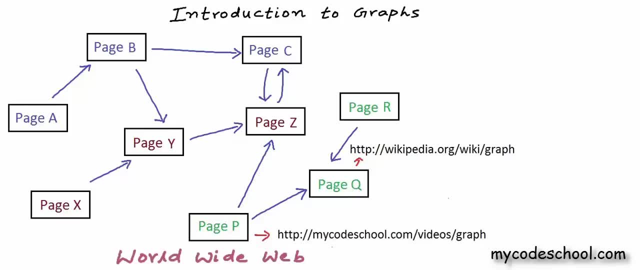 you cannot click on a link and come to page P Connection here is one way, and that's why we have drawn a directed edge here. Okay, now, once again, if we are able to represent web as a directed graph, we can apply standard graph theory algorithms to solve problems. 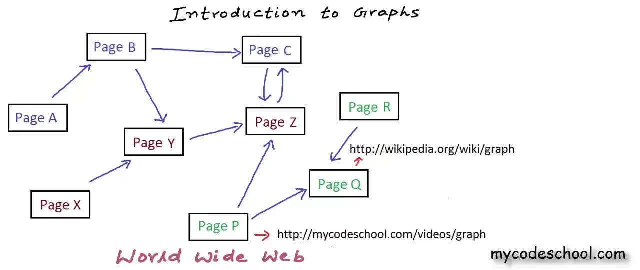 and perform tasks. One of the tasks that search engines like Google perform very regularly is web crawling. Search engines use a program called Web Crawler that systematically browses the world wide web to collect and store data about web pages. Search engines can then use 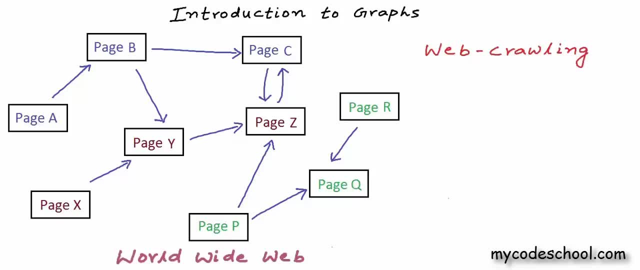 this data to provide quick and accurate results against search queries. Now, even though in this context we are using a nice and heavy term like web crawling, Step crawling is basically graph traversal, or, in simpler words, act of visiting all nodes in a graph And no prizes for guessing that there are standard algorithms for graph traversal. 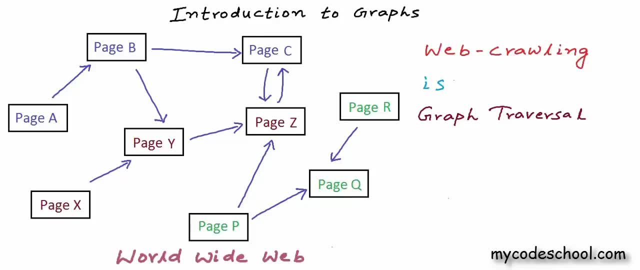 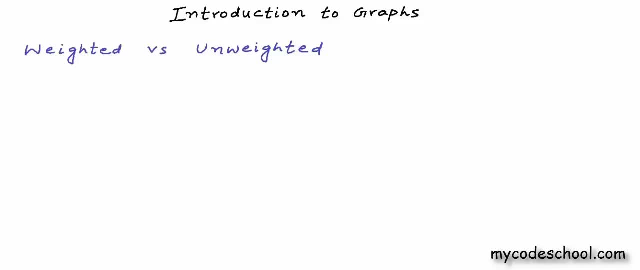 We will be studying graph traversal algorithms in later lessons. Okay, now, the next thing that I want to talk about is concept of a weighted graph. Sometimes in a graph, all connections cannot be treated as equal. Some connections can be preferable to others, Like, for example, we can represent intercity road network, that is, the network of highways. 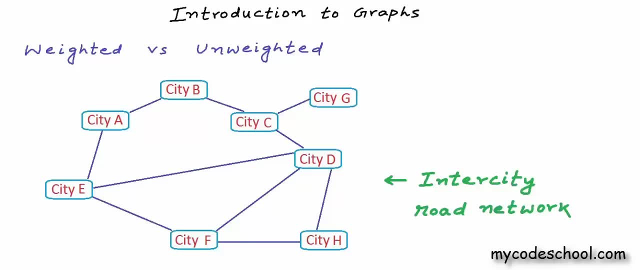 and freeways between cities as an undirected graph. I am assuming that all highways would be bidirectional. Intracity road network, that is, road network within a city, would definitely have one way roads, and so intracity road network must be represented as a directed graph, but intercity. 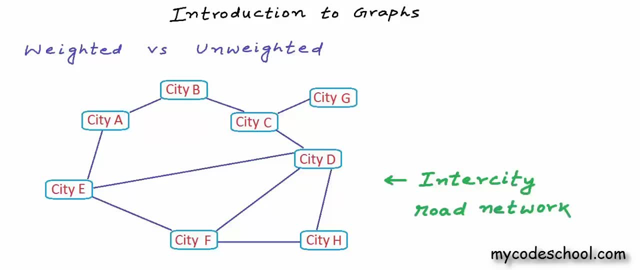 road network, in my opinion, can be represented as an undirected graph. Now, clearly, we cannot treat all connections as equal here. Roads would be of different lengths and to perform a lot of tasks to solve a lot of problems, we need to take length of roads into account. 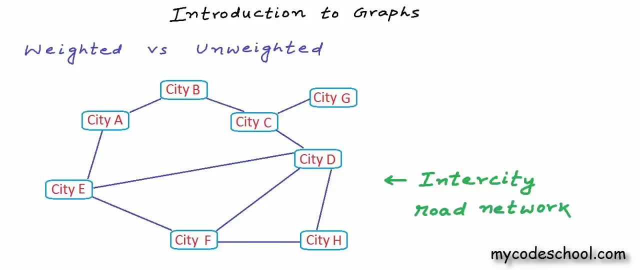 In such cases we associate some weight or cost with every edge. We label the edges with their weights. In this case, weight can be length of the roads. So what I will do here is I will just label these edges with some values for their lengths. 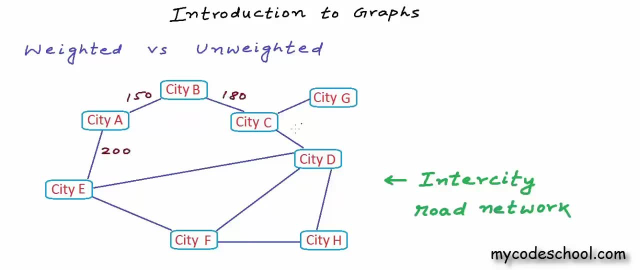 Okay, Let's say these values are in kilometers and now edges in this graph are weighted and this graph can be called a weighted graph. Let's say, in this graph we want to pick the best route from city A to city D. Have a look. 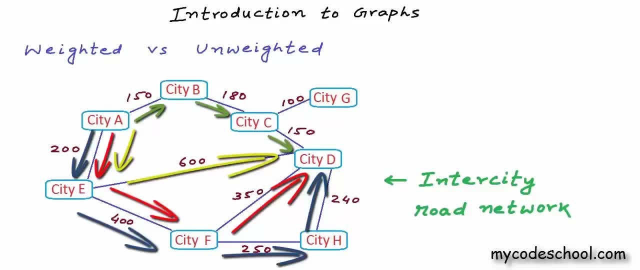 at these four possible routes. I am showing them in different colors. Now. if I would treat all edges as equal, then I would say that the green route through B and C and the red route through E and F Are equally good. both these paths have three edges, and this yellow route through E is the. 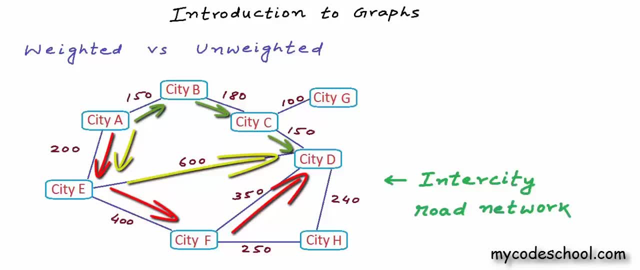 best because we have only two edges in this path, But with different weights assigned to the connections. I need to add up weights of edges in a path to calculate total cost. When I am taking weight into account, shortest route is through. B and C. Connections have different weights and this is really important here in this graph. 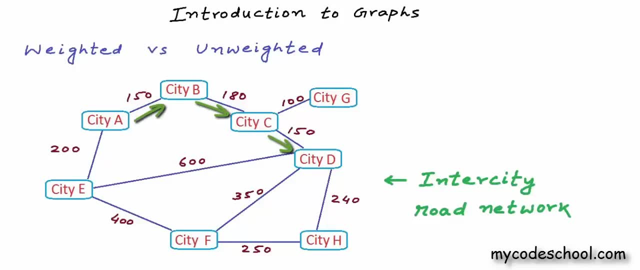 Actually, we can look at all the graphs As weighted graphs. An unweighted graph can basically be seen as a weighted graph in which weight of all the edges is same and typically we assume the weight as one. Okay, so we have represented intercity road network as a weighted, undirected graph. 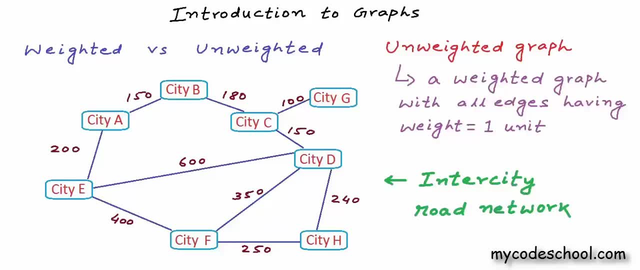 Social network was an unweighted, undirected graph and world wide web was an unweighted, directed graph, And this one is A weighted, undirected graph. Now, this was intercity road network. I think intracity road network, that is, road network within a city, can be modeled as a